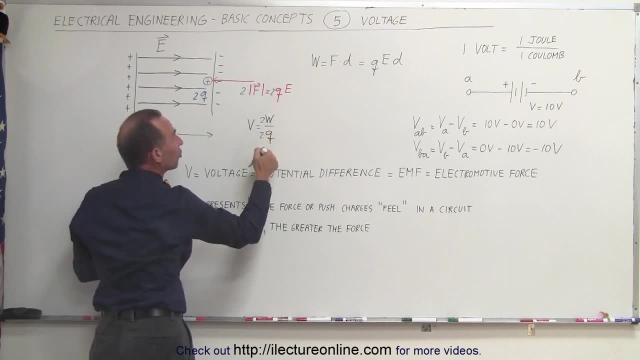 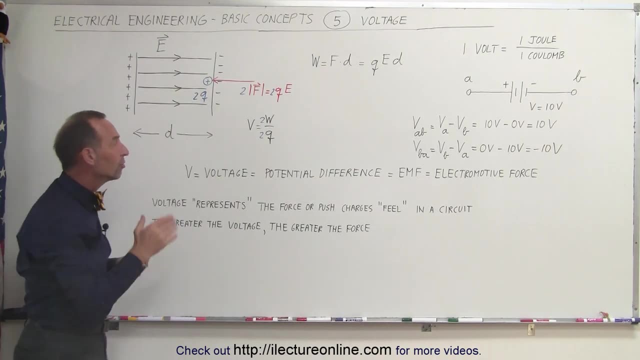 therefore, twice the work and we would have twice the charge. And you see that that ratio will always be the same, regardless as to the size of the charge that we use. So it's always the ratio of the amount of work done divided by the charge used, and regardless how big we make that charge, that ratio is always the same. 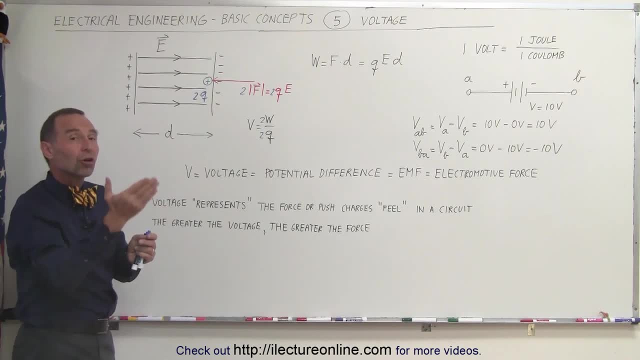 and that is then defined as the voltage. It's the work done to get a charge across from the left side to the right, or from the right side to the left side, in this case from the negative charge to the positive charge, through an electric field divided by the charge. 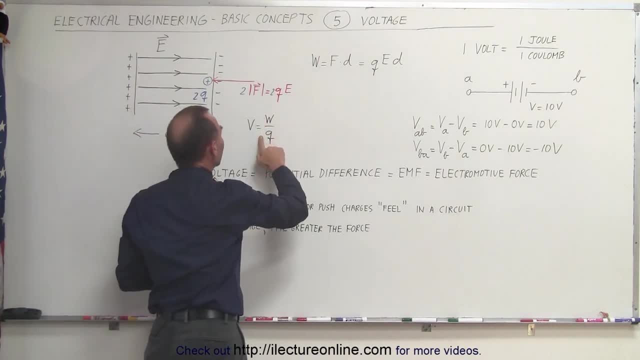 required If we plug in, if we get rid of these twos again right here, if we plug in what work is equal to? we can see that the work is equal to qe times d divided by the charge q. The q's cancel out. 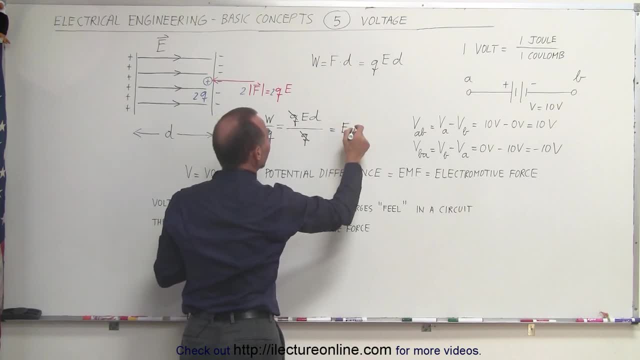 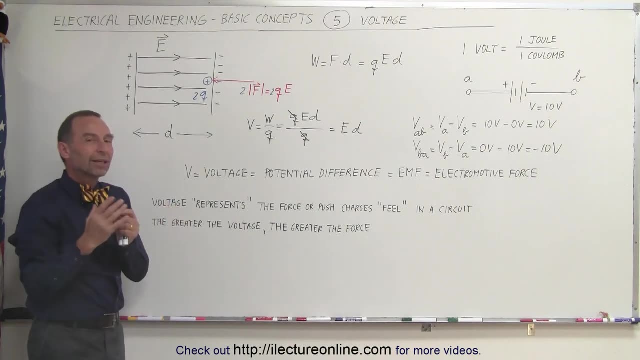 which means that the voltage, then, is defined as the strength of the electric field times the distance between the left side and the right side of that field. The voltage can be thought of in two ways. It's equal to the amount of work we need to do to get a charge across from the electric field. 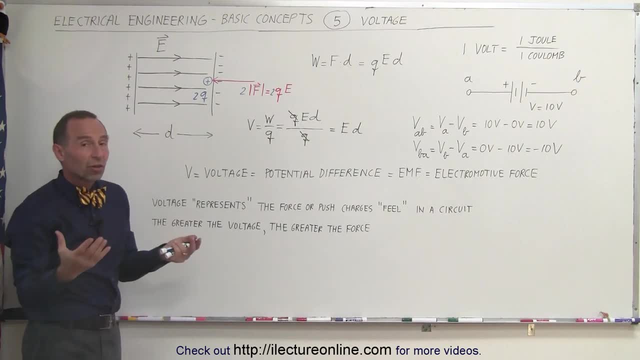 A charge moved through an electric field, divided by the size of the charge, or simply the potential difference, or voltage, is equal to the strength of the electric field times the distance. Now a volt is defined, therefore, as a joule per coulomb. Remember. 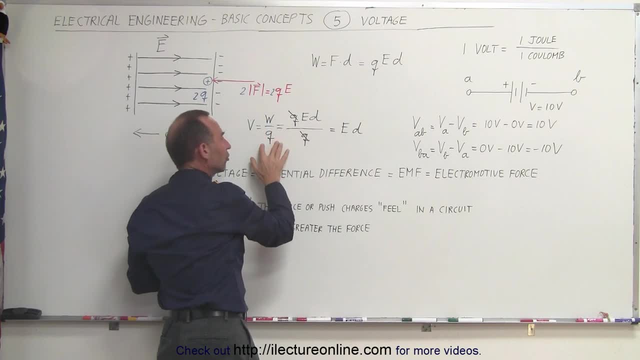 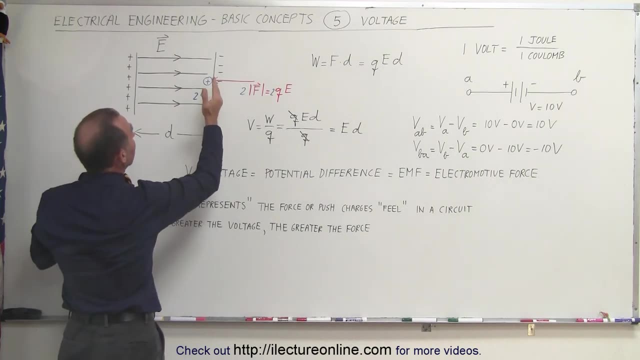 it's work over charge. Work is in joules. Charge is in coulombs, So a volt is defined as a joule per coulomb. In other words, if we have one coulomb of charge and it takes one joule of work to get it across. 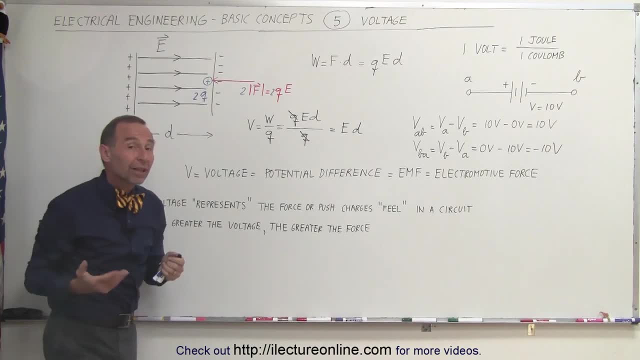 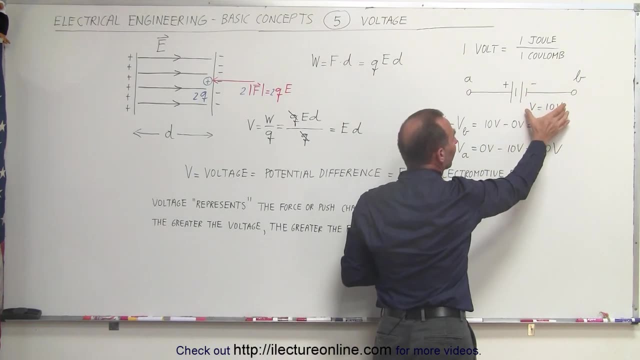 That means that the voltage between those two plates is equal to one volt. That's how we wanna look at it. If we have a battery and we have a positive end of the battery and we have a negative end of the battery and the volts across the battery is 10 volts. 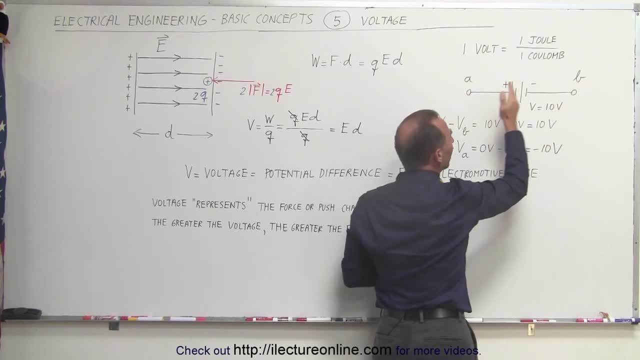 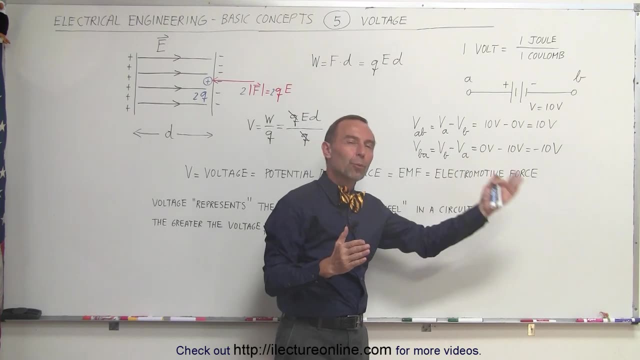 we can say that the voltage at A is 10 volts higher than the voltage at B. So sometimes we talk about potential difference or voltage difference. It is how much more volts we have on one side compared to the other side. In this case, A is 10 volts higher than B. 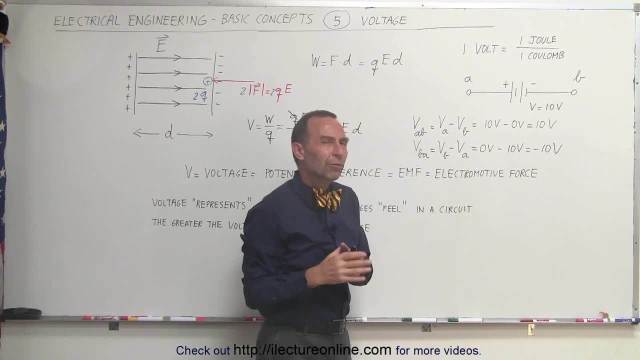 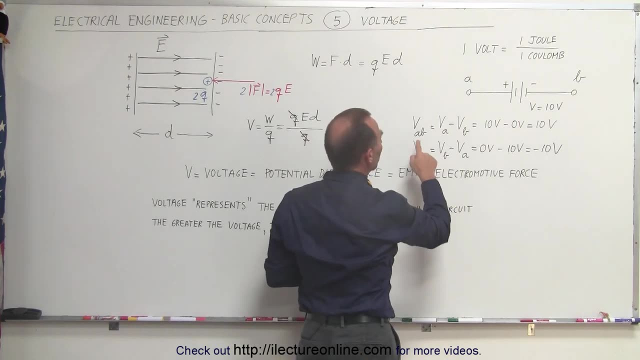 B could be 100 volts, then A would be at 110 volts. Whenever we talk about the voltage of a battery, we really talk about the difference in the voltage, or the potential difference, This case, when we talk about volts from A to B. 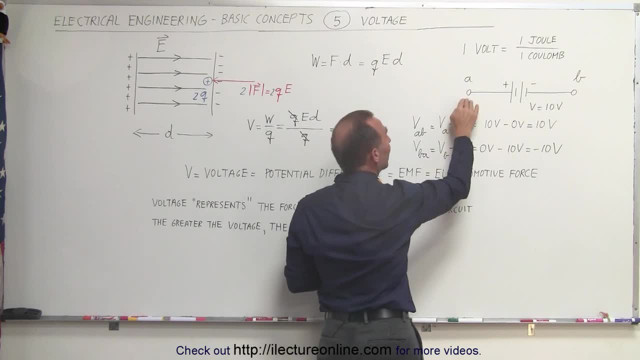 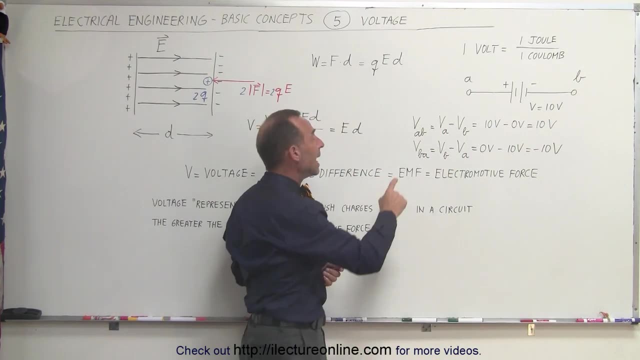 that is equal to volts at A minus volts at B. Since A is bigger than B, it'll be 10 volts minus zero volts, which is a 10 volt difference. But if we talk about VBA, this is equal to V at B. 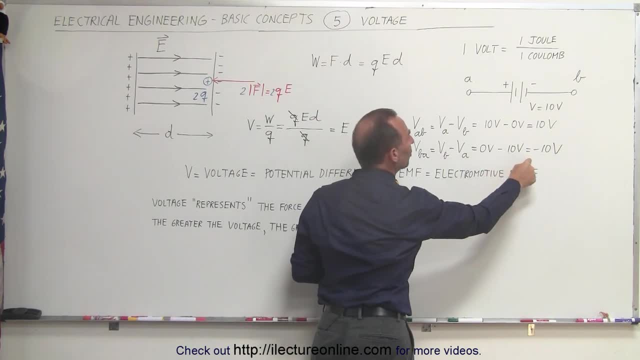 minus V at A, which is equal to zero volts. minus 10 volts is equal to minus 10 volts. When we go from B to A, we increase in voltage by 10 volts. If we go from A to B, we decrease by 10 volts. 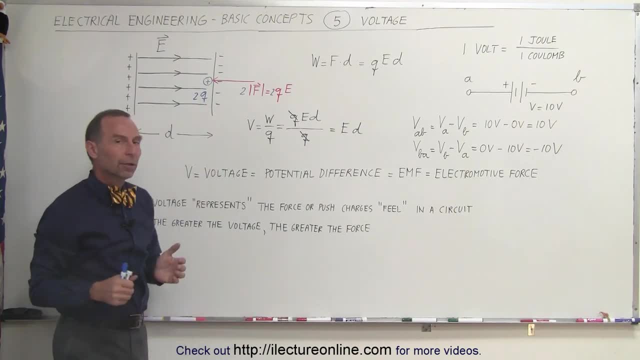 That's a negative voltage direction. Another way of looking at voltage: V voltage is equal to the potential difference. Potential difference means a voltage difference between two points on the circuit. Sometimes it's also called the EMF or the electromotive force. 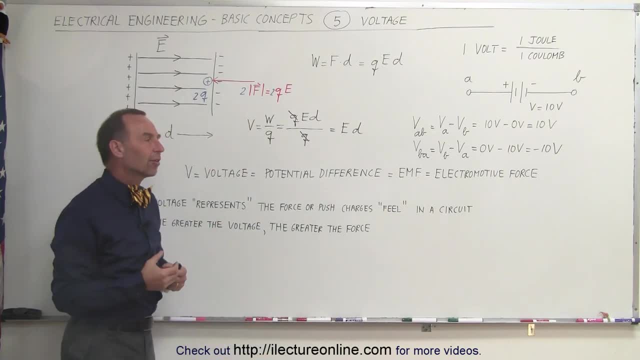 And one of the reasons why we think about it as the electromotive force is because voltage is really the amount of volts you have on a circuit or in a battery determines how much push charges feel to move through the circuit. Another way of looking at voltage is to say: 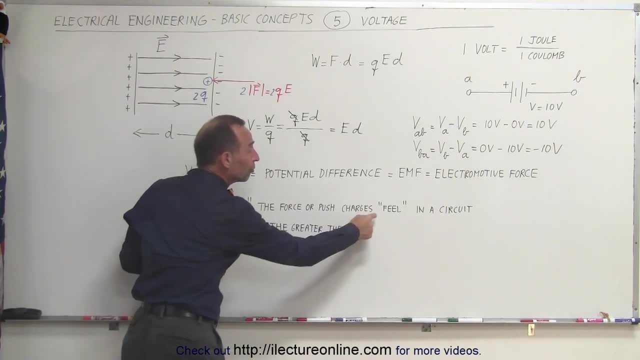 that the voltage represents the force or push charges feel. Of course charges don't really feel anything, but if you think about it, if you're a charge and there's a voltage difference there, you're going to feel a push to the circuit. 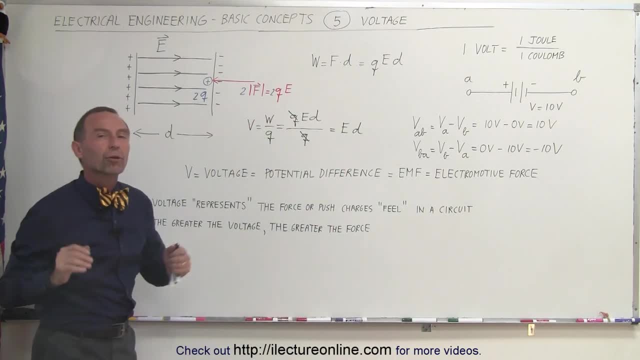 It's going to feel as if you're being pushed through that circuit by the voltage difference. The bigger the voltage difference, the bigger the voltage across that battery. the more push that charge is going to feel. The greater the voltage, the greater the force. 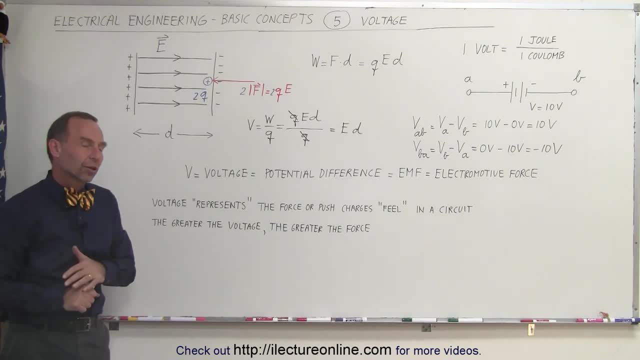 or the push that the charges feel inside the circuit, The bigger the potential difference, the greater the force, the more push to get the charges around the circuit And that's why very large voltages can be very dangerous, because large pushes can actually become. 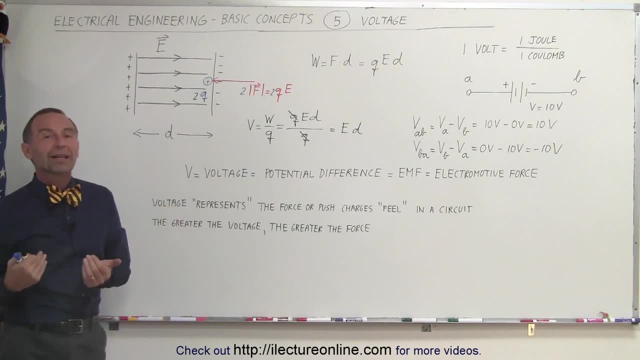 dangerous when you get near that. Charges may get pushed through your body if you touch the circuit and if the potential difference of the voltage is very large. Again, voltage, think of it as that thing that pushes charge through circuits. The bigger the voltage, the bigger the push. and that's a good place to start.